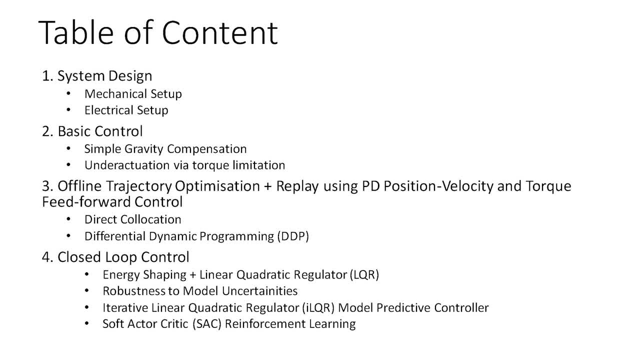 and electrical setup of the pendulum, show basic control methods before talking about offline trajectory optimization, feedforward and closed-loop control. 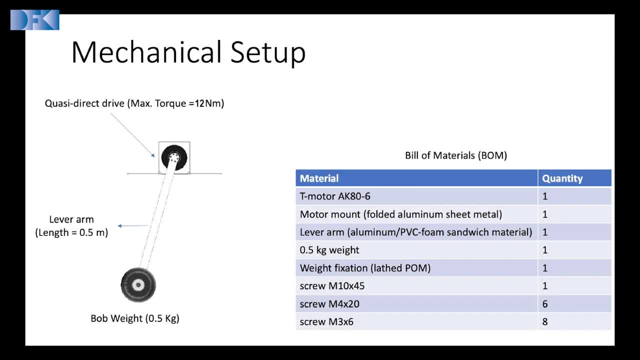 The pendulum consists out of four main components. A 500g weight, a 0.5m swingarm, a motor and motor mount. The selected motor is a quasi-direct drive BLDC motor with a gear ratio of 1 to 6 and a maximum peak torque of 12 Nm. 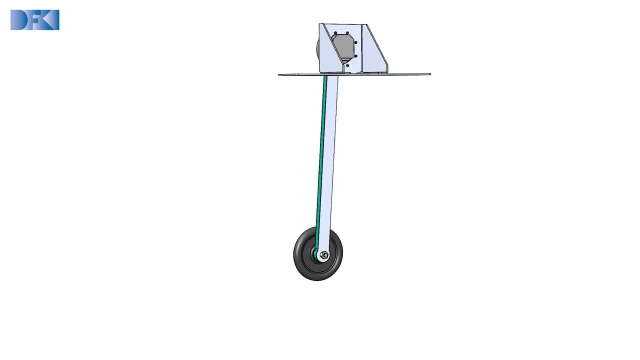 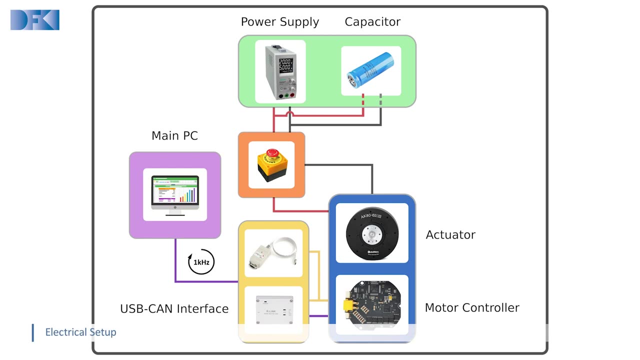 A bill of material including all mechanical parts together with the CRD files of the assembly is included in the repository. Either a power supply or a battery pack can be used to power the pendulum. The pendulum is a very powerful and powerful actuator. The capacitor absorbs voltage spikes caused by the back-MF whenever the motor is decelerating. For safety reasons, an emergency stop cutting off the actuator from both, power supply and the capacitor is required. The BLDC motor we use comes with an integrated motor controller board. The motor controller board handles phase commutation at high frequency rates, usually between 20 and 40 kHz. Higher level commands like desired position, velocity or torque are sent from an external PC via CAN bus to the motor controller with a frequency up to 1 kHz. Most consumer PCs do not feature CAN ports. Hence, an additional UR2CAN adapter is needed. 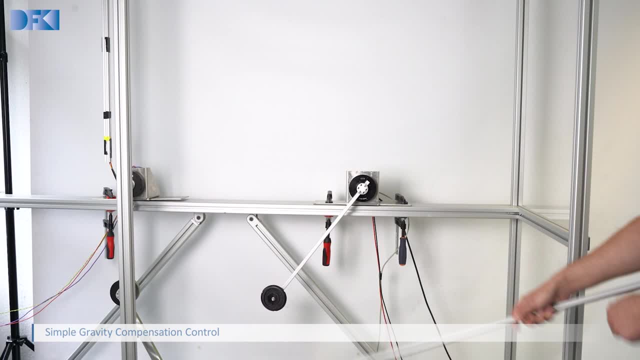 Let's begin with a simple gravity compensation controller to showcase torque-based control. Knowing the weight attached to the rod and the length of the rod, the controller is able to cancel out the gravity vector, basically allowing the weight to freely float in space. 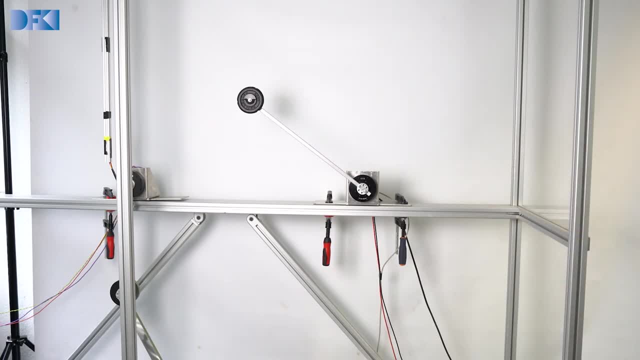 Once the controller is switched off to the weight instantly falls down, underlining low friction and back-drivability of the system. 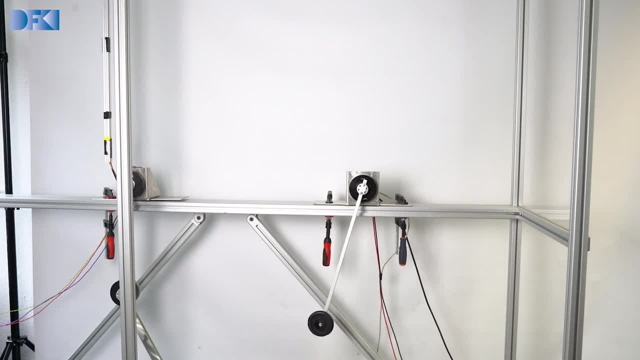 The pendulum approximately requires 2.5 Nm of torque to lift the weight non-dynamically in the top position. Given 1 Nm of torque, instead the weight is only lifted by around 20 degrees and fails to swing up, as we can observe. All subsequent controllers aim to lift the weight into the top position within the torque limitation of 1 Nm. 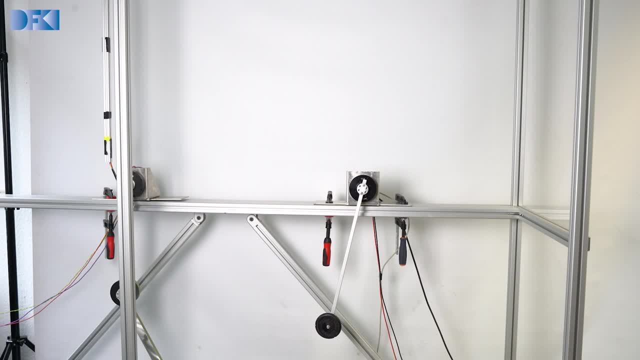 This task belongs to the research field of underactuation in robotics, where the performance of robotic systems can be enhanced above given torque limitations by exploiting the natural dynamics of a task. 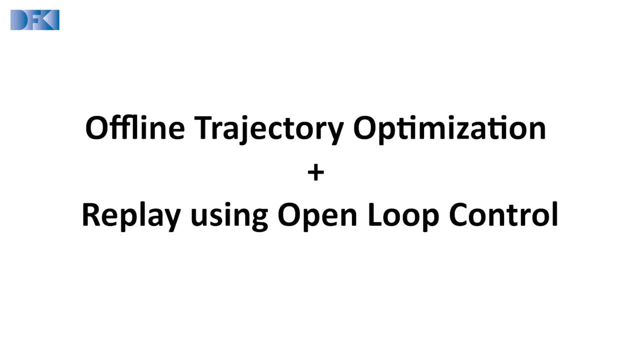 Using a physical model of the system, a swing-up trajectory has been optimized offline via direct collocation, and is later executed in open-loop control on the real pendulum. Direct collocation is a non-linear optimization technique in which the swing-up trajectory is controlled by an open-loop control on the real pendulum. Direct collocation is a non-linear optimization technique in which the swing-up trajectory is controlled by an open-loop control 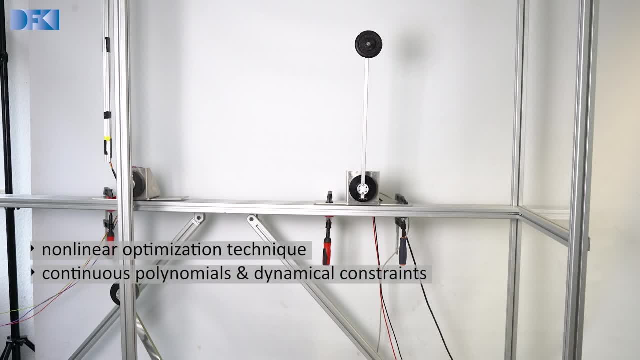 on the real pendulum. A state trajectory is split piecewise into a continuous polynomials, and dynamic constraints are imposed on intermediate points, the so-called collocation points. The optimal solution is required to satisfy the conditions of optimality only at these intermediate points, which significantly decreases computation time to derive a control policy. 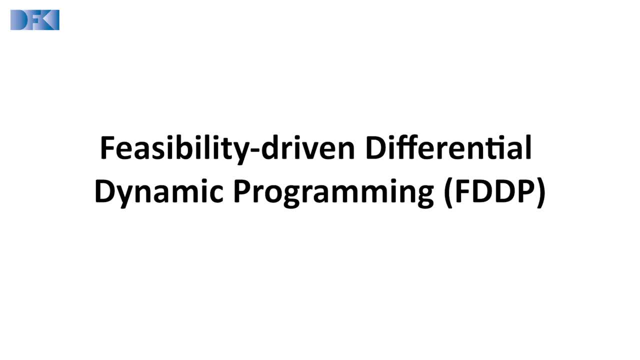 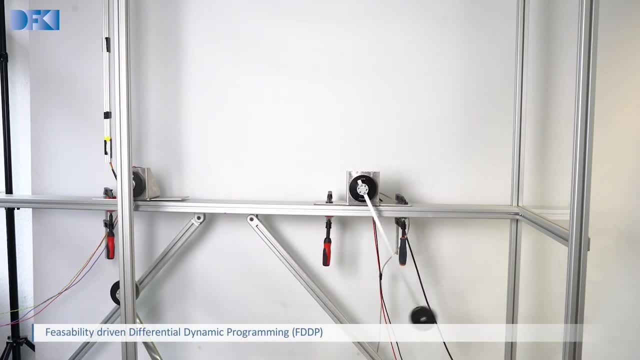 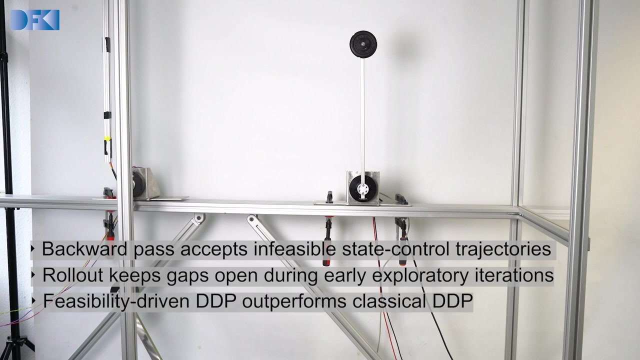 Another solver as called DDP explicitly handles the geometric structure of control problems, including elements of SE3, but has pure globalization strategy and struggles to handle infeasible warm starts. A new solver, namely feasibility-driven differential dynamic programming, addresses these issues by adding two modifications to the classical DDP algorithm. First, the backward pass also accepts infeasible state-controlled trajectories. Second, the row load keeps the gaps open during early exploration iterations. These modifications result in a superior optimal control solver that outperforms classical DDP 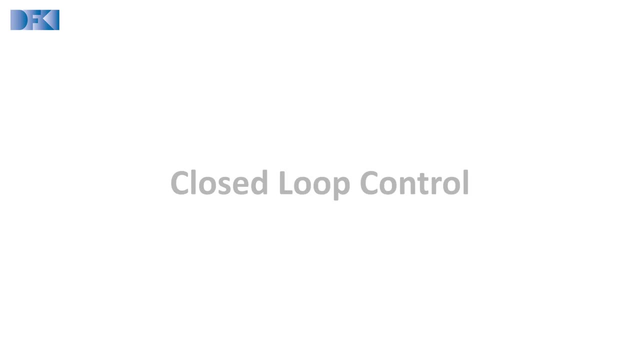 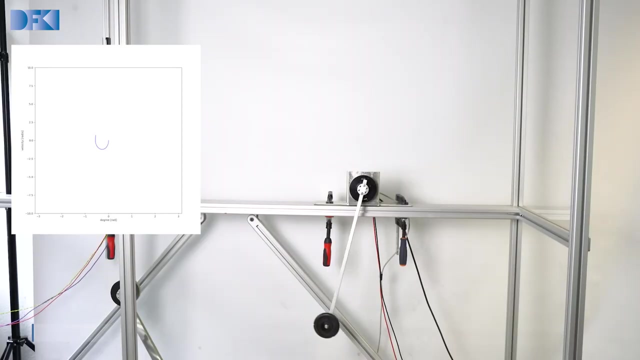 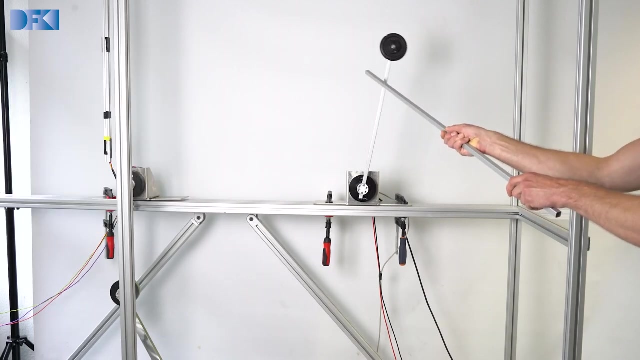 through faster computation times. The energy-shaping controller always pushes the pendulum towards the upright position, where the system encounters its maximum potential energy and the kinetic energy is zero. If the total energy of the system is smaller than the potential energy in the upright position, the controller adds energy to the system by applying torque in the direction of motion. And conversely, if the total energy is higher than the potential energy in the upright position, the controller subtracts energy from the system by outputting torque in the opposite direction. 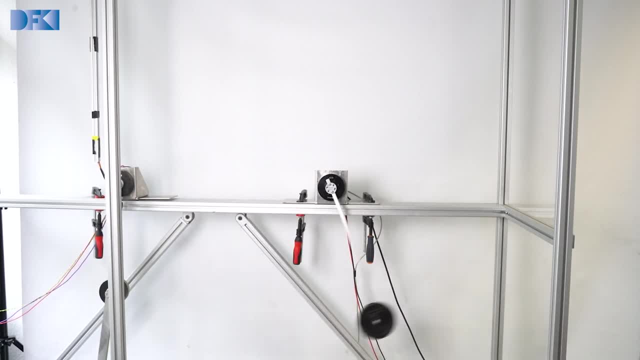 The simplicity of energy-shaping controller makes it inherently stable to model uncertainties. It manages to achieve a swing-up of a weight of 1 kg, although the underlining model expects only half a kilogram, and even can recover from a double swing. 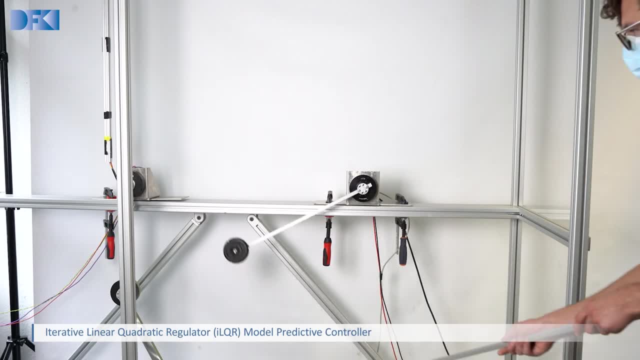 The iterative linear quadratic regulator is an extension to the LQR controller. While the standard LQR controller linearizes the dynamics at a given state and assumes that these linear dynamics are globally valid,